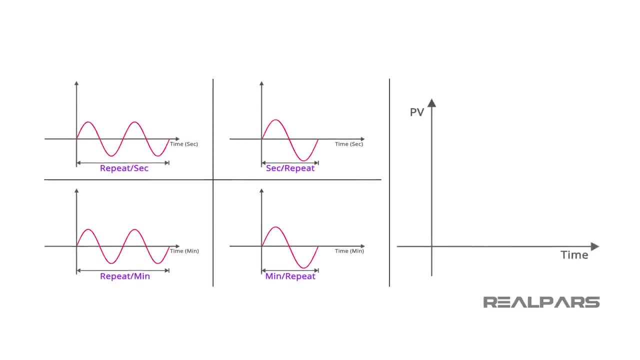 Essentially, regardless of the measurement type, the integral is the sum of all of the values reported from the signal captured, from when you started counting to when you completed counting, or the area under a plotted curve. This parameter can be called Ki, Ti or others. 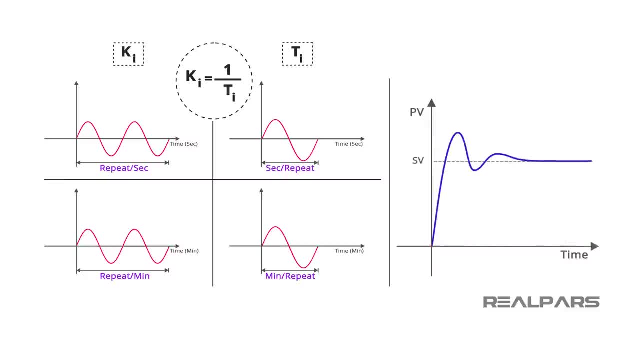 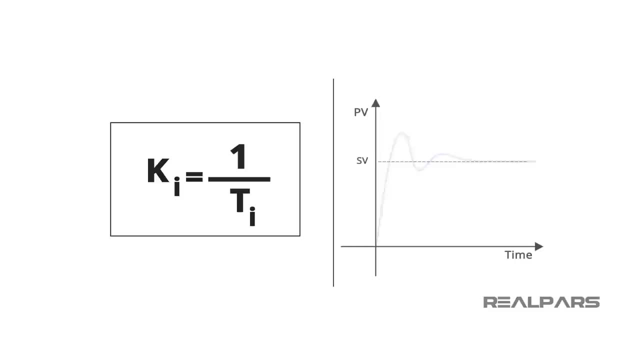 This parameter determines how fast the steady-state error is removed. Because of the different measurements, this parameter may not be as intuitive to adjust. Briefly, smaller values in minutes per repeat measurements will create larger integral action where larger values in repeats per minute measurements. 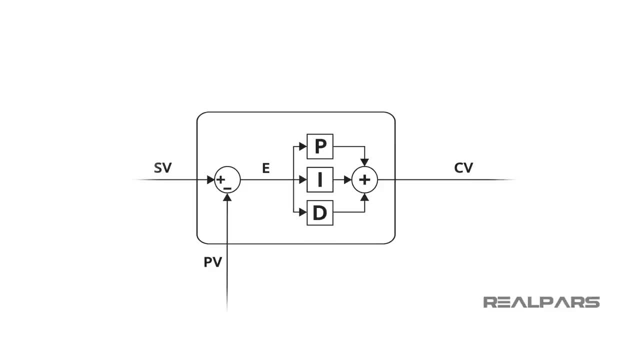 will create larger integral action. Derivative or D constant units are typically seconds or minutes. The purpose of derivative constant is for predicting change. The derivative action acts of the rate of change measured in the process variable. The value of this parameter basically means: 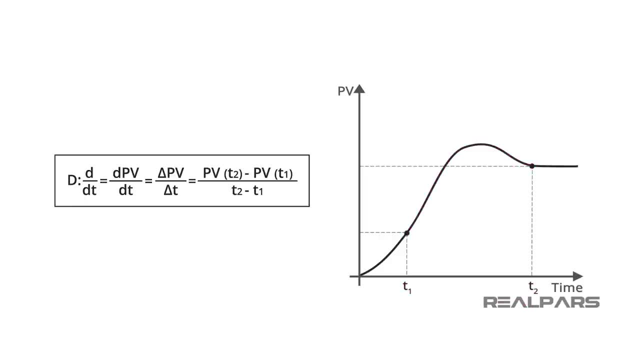 how far in the future you want to predict the rate of change. This parameter can help to create a faster response in your loop and a better performing loop as well. However, since the derivative term is measuring the rate of change in the process variable, 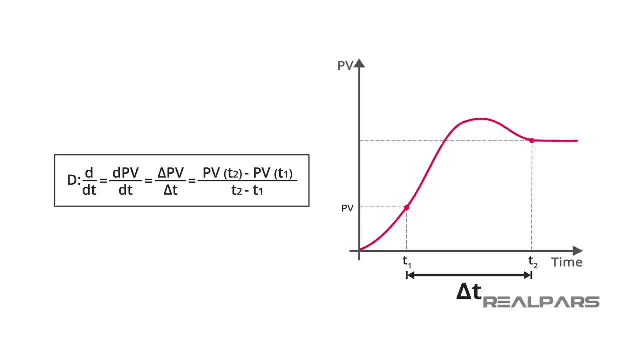 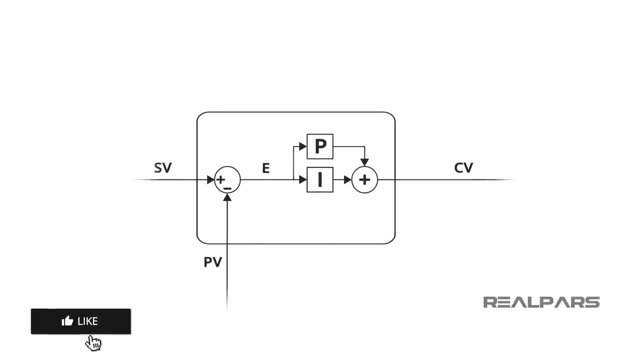 the process variable must be a very clean signal, meaning no noise within the signal. For that reason derivative terms are not often used in controls. The most commonly used controller is the PI. Most processes can be well served with this type of control. 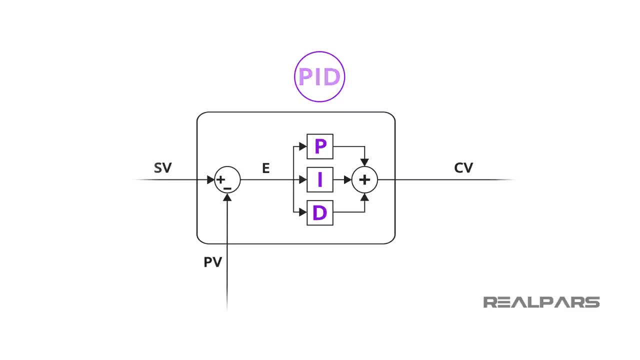 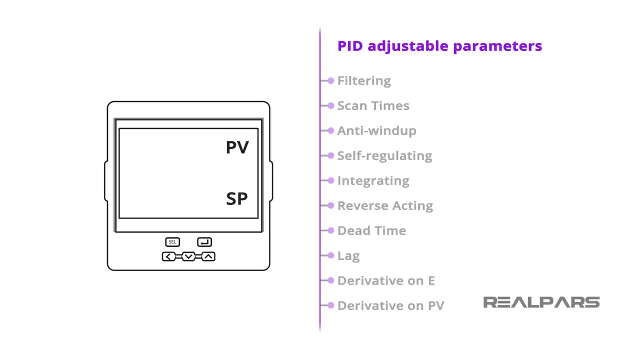 P and PID controllers are occasionally used, while PD controllers are rarely used. PID controllers are very sophisticated devices with likely many adjustable parameters. The process and algorithm types can also vary. Other parameters to research for PID controllers are series, ideal and parallel algorithms, filtering, scan times, anti-windup. 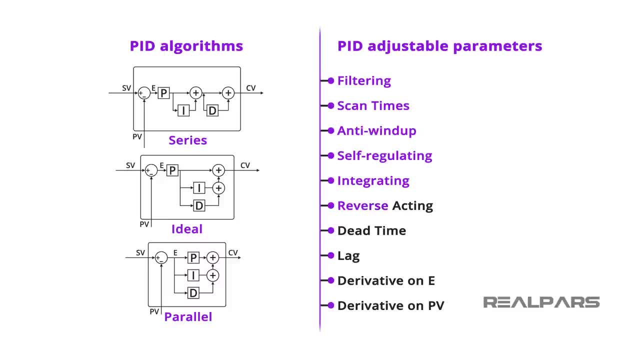 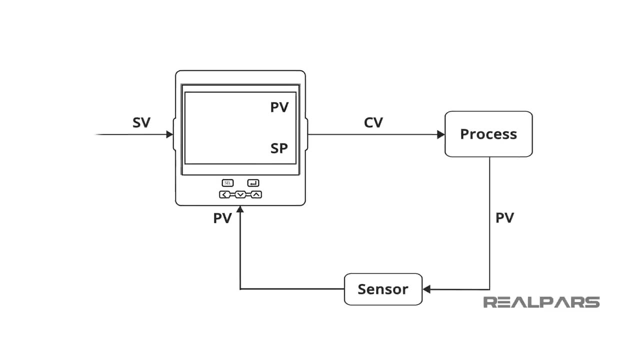 self-regulating versus integrating processes, reverse acting, dead time lag, derivative on E or derivative on PV, just to mention a few, With no difficulty in tuning the most basic of PID loops, these parameters, which are more advanced than this basic tutorial. 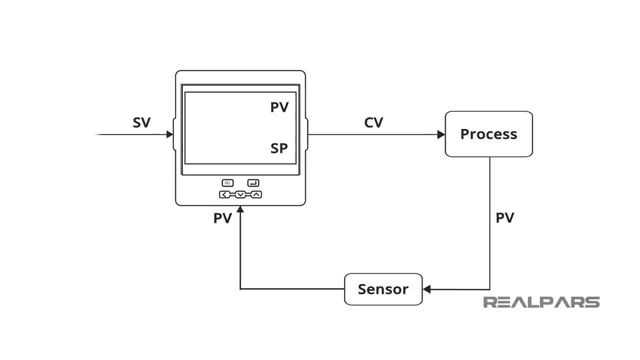 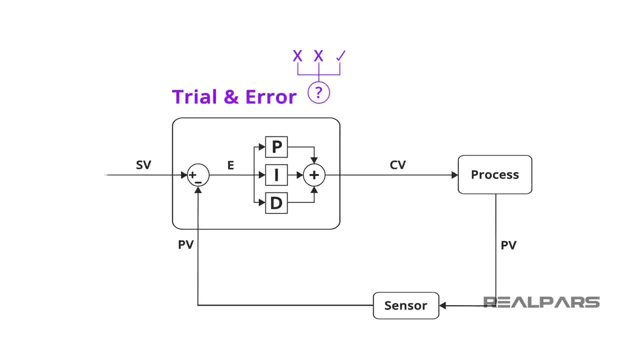 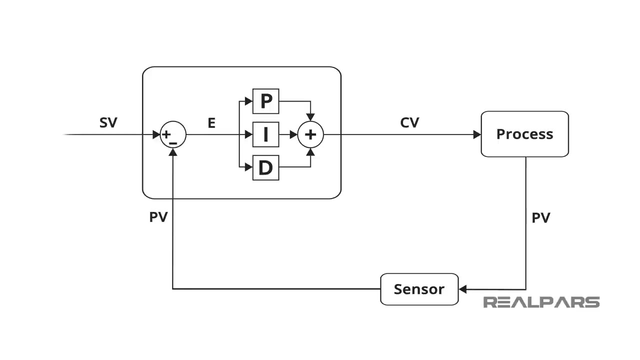 are better left for future lessons or self-exploration. There is a science to tuning a PID loop, but the most widely used tuning method is trial and error. There are other methods that require a multi-step process to determine where your numbers should be. 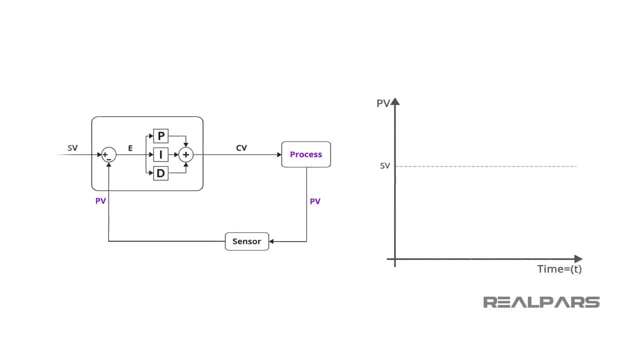 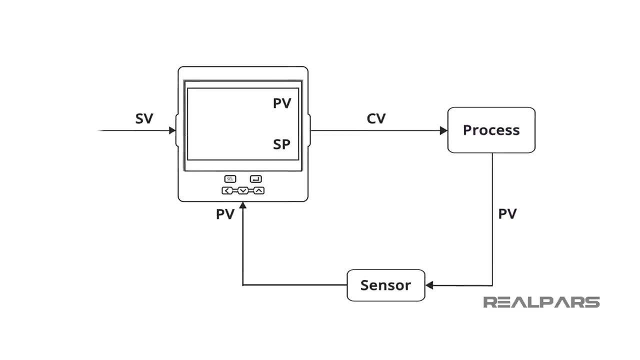 Your goal is to control the process when plotted in a trend as a nice, even trend line with minimal oscillation. The first step in tuning your controller is to determine just how much adjustment you can make without serious implications to the process. Talk to the plant personnel. 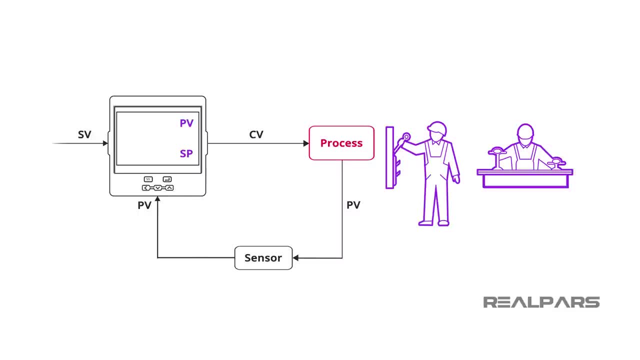 If adjusting the parameters of the PID controller will not have an adverse reaction, then you can begin your adjustments. If the effects will be detrimental, you must take a more measured approach, Obviously depending on whether this is a new installation or an existing plant. 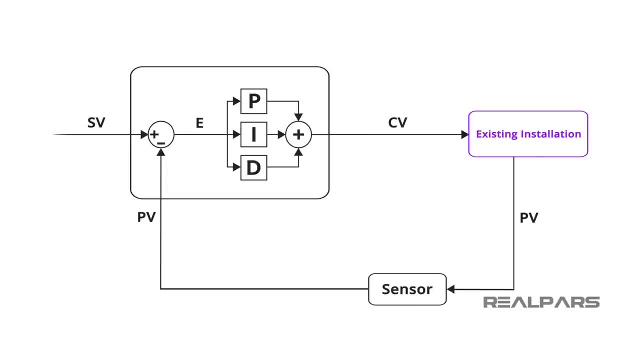 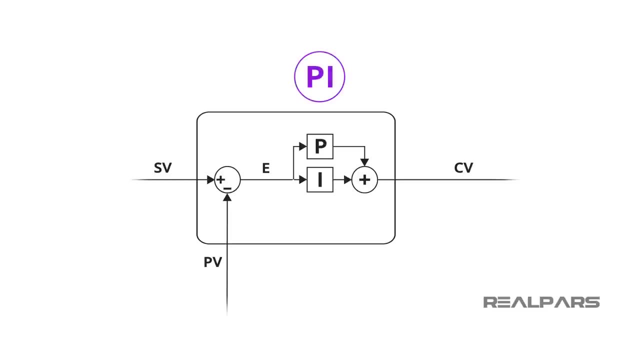 your approach will be different. In existing installations, you are just looking to tweak values and create a more stable process. Because the PI controller is the most widely used, we will only be adjusting those parameters As we have discussed the differences and measurements in the PID terms. 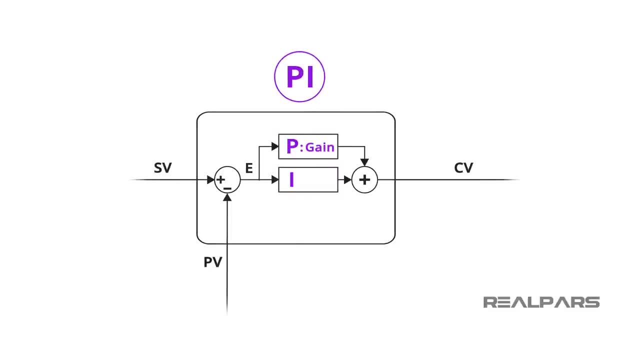 for this tutorial. we are going to standardize on gain and repeats per minute, To just jump right in. if your process variable changes quickly and changes to your control variable, you will start with a low gain, possibly as low as 0.1,. 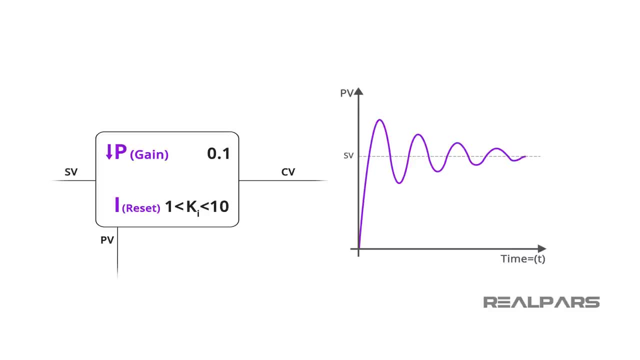 while adjusting your reset, between 1 and 10 repeats per minute. Conversely, if the process variable changes slowly, start with higher gains and lower resets, somewhere between 2 and 8, and 0.05 and 0.1.. Adjust only one parameter at a time. 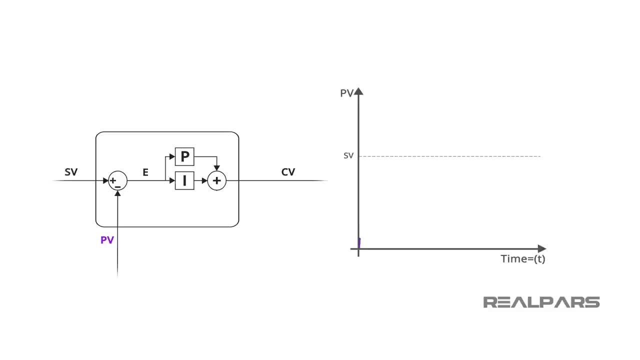 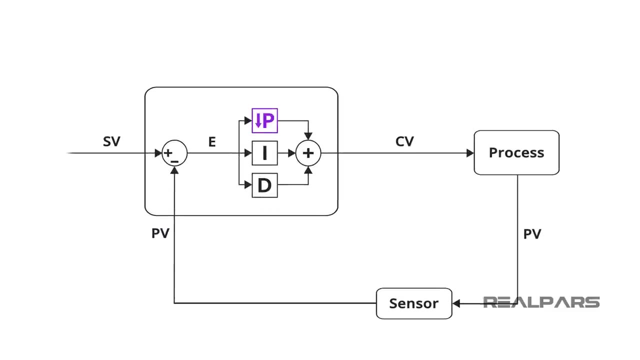 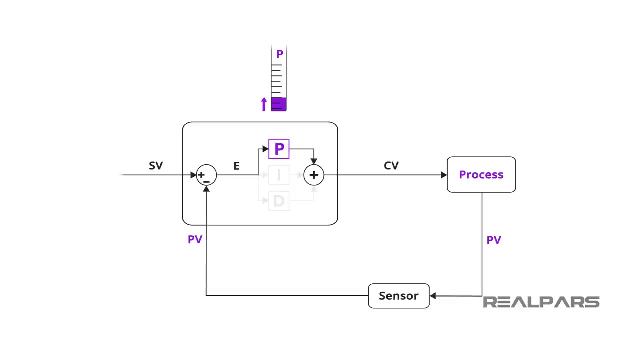 and observe the results. Continue in this vein until you have achieved a stable process. A more measured approach is to start with a low gain with integral and derivative disabled. Watch the process and begin incrementally adjusting the gain by doubling the value When the process begins to oscillate.